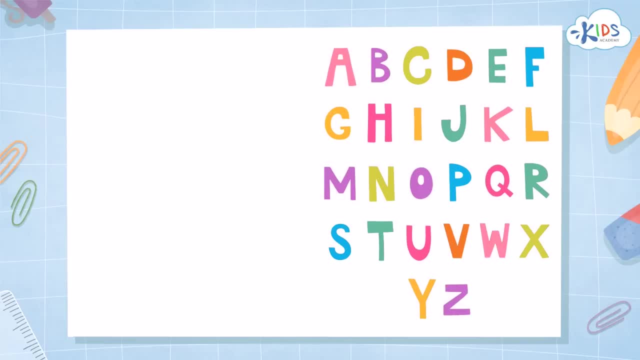 the letters of the alphabet Letters are written in a certain order to spell different words. Listen to the word dog. The word dog is written with three letters: D O G, D, D O G, O, A, G, G, D O G, Dog. Let's read together: Dog, Very good. Listen to the word cat: The. 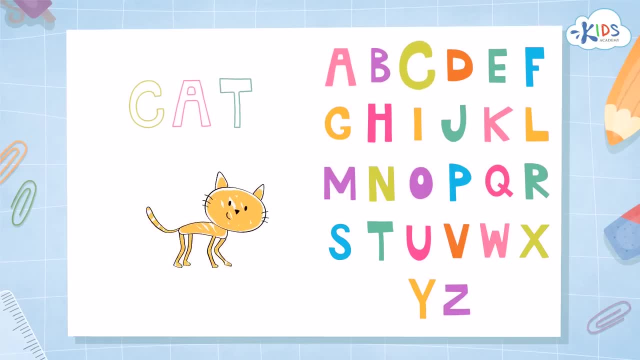 word cat is written with three letters: C A T C. C A A T, T, C A T, Cat. Can you read this word Cat? Well done, Listen to the word mop. 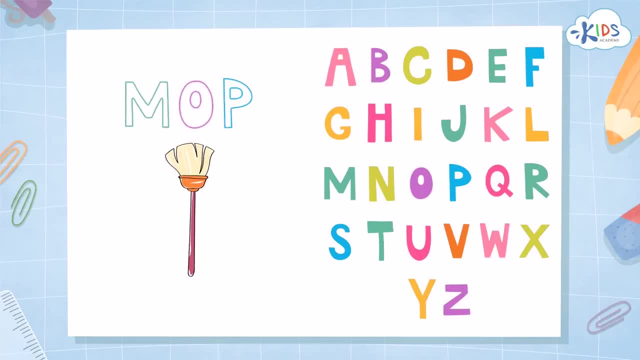 The word mop is written with three letters: M, O, P, M, M, O, A, P, P, M, O, P, Mop. Let's read this word together: Mop, Excellent, Now you can practice. 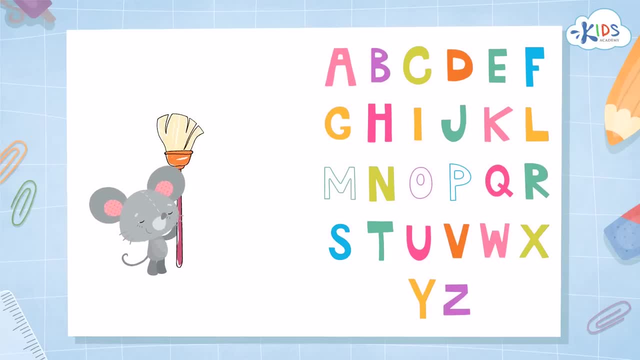 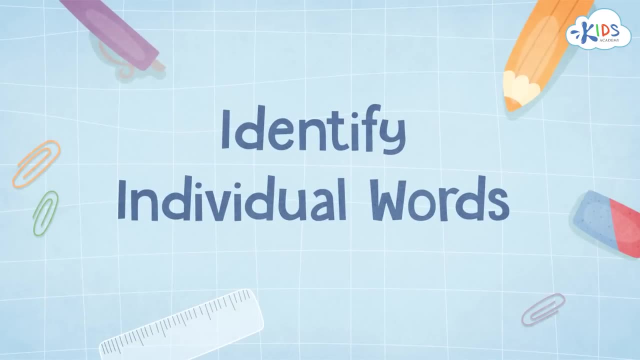 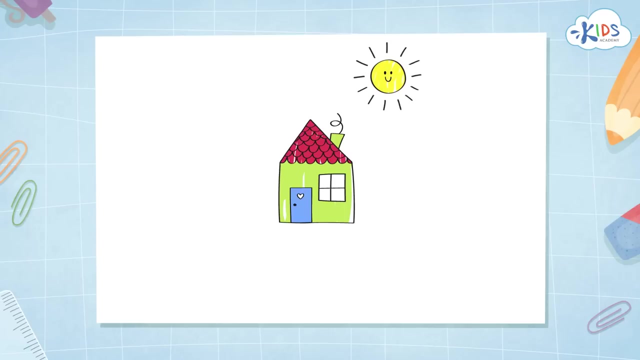 finding words that are written out on your own. See you later, Hi everyone. In this lesson you will learn why we put spaces between words when we write. Look at this sentence. The sun is hot. Do you see that there is a space between each word? We can see that there are four words in the 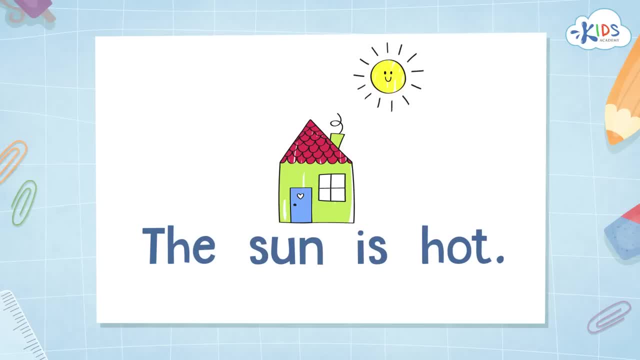 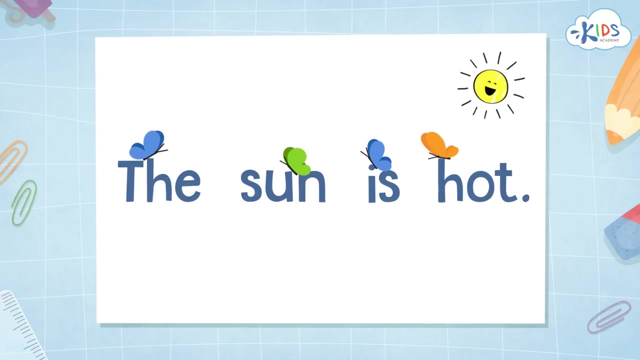 sentence. Let's count together One, two, three, four. Whenever you write, you must put a space between every word. If you don't put spaces between your words, you will not be able to write. We have a long list of words. People can't tell where one word ends and another starts. That would 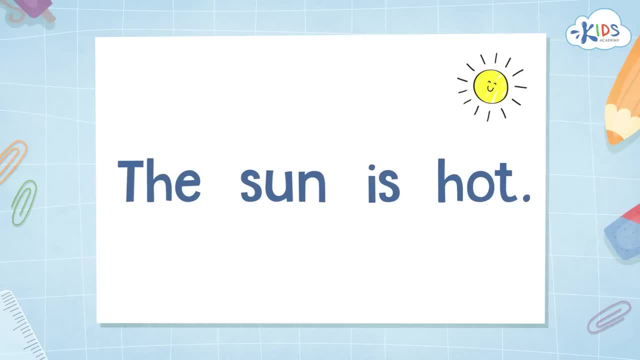 make it very hard to read. Much better now. What is wrong with this sentence? Yeah, There are no spaces between the words in this sentence. Can you see how this makes it very hard to read? It is much easier to read when we put spaces between the words. Now let's read together. Can you see how this? 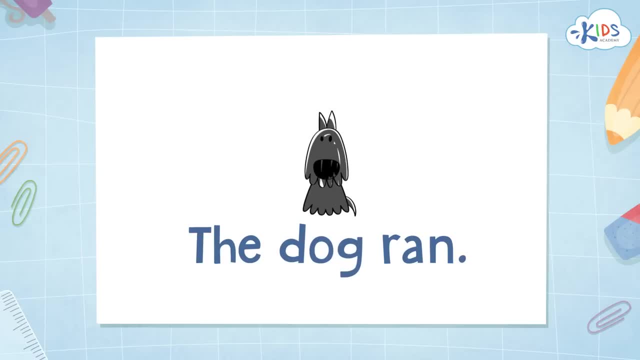 makes it very hard to read. It is much easier to read when we put spaces between the words. the dog ran. there are three words in this sentence. let's count together one, two, three. let's take a look at another sentence. I see the cat. how many words. 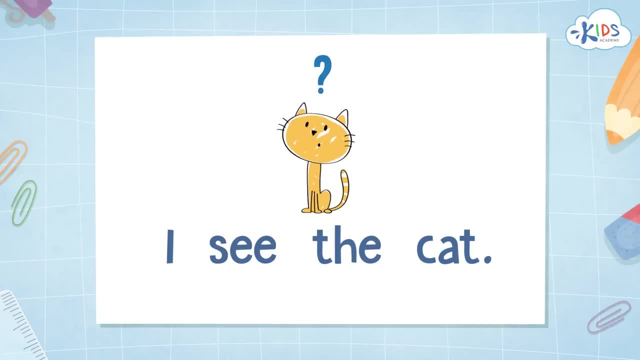 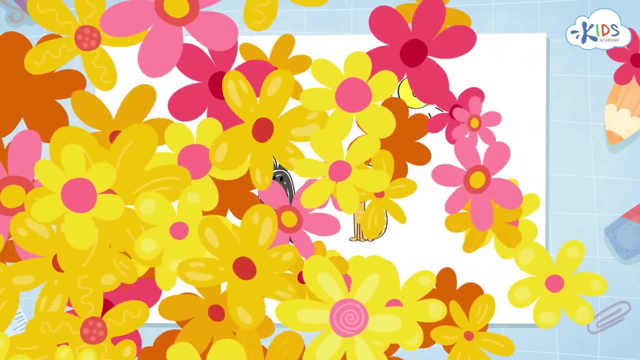 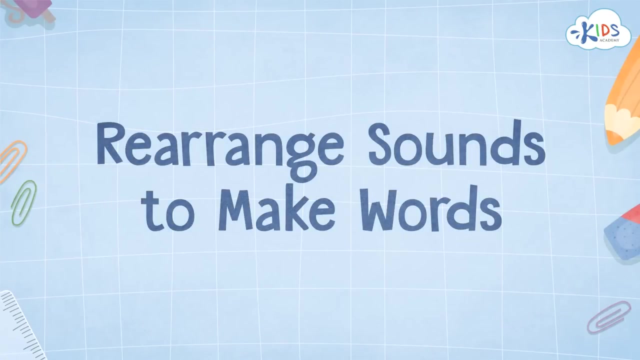 are in this sentence. there are spaces between each word. this helps us see that there are four words in the sentence. let's count together one, two, three, four. well done, now you can practice finding spaces between written words. bye, hi, everyone. in this lesson, you are going to learn how to put sounds in order to make 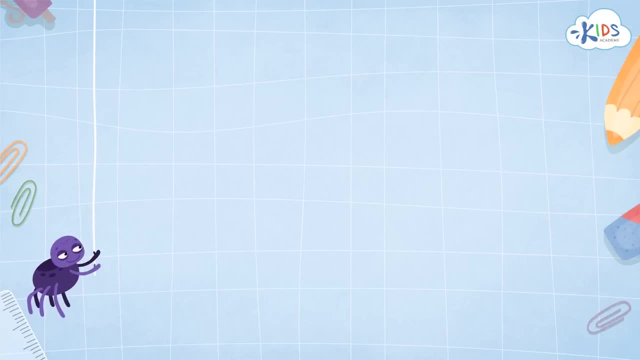 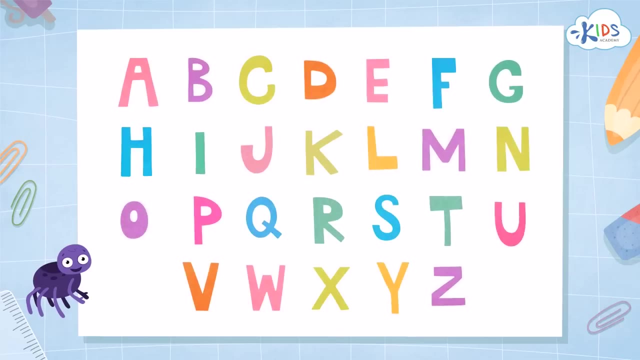 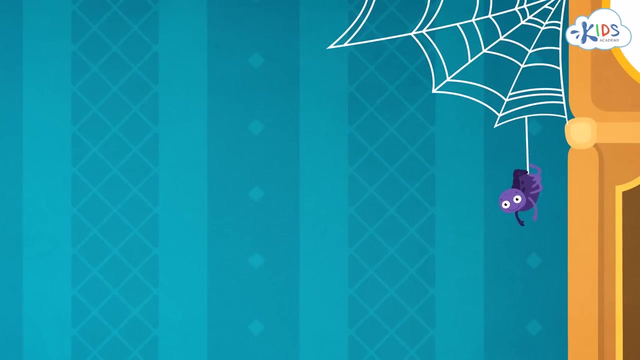 words. every word that you hear in a sentence should be in the same order as the words here can be written down. to write words we use the letters of the alphabet. letters are written in a certain order to spell different words. look, d-o-g. dog, see at cat, the spider and the song: the itsy-bitsy spider made a spider. 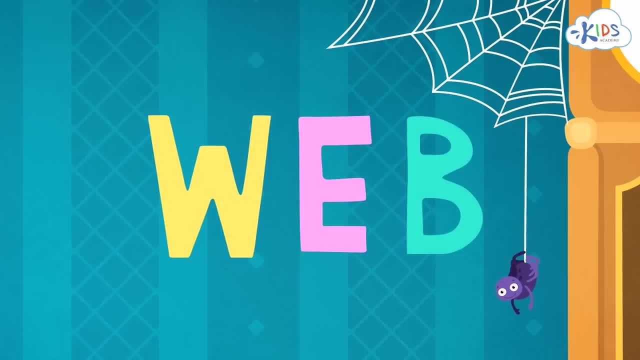 web. The word web is written using three letters of the alphabet. It starts with a W, which makes the W sound. The word web has the letter E in the middle. The letter E makes the E sound. The letter B is at the end of the word web. B makes the B sound. When we put all of the letter sounds together. 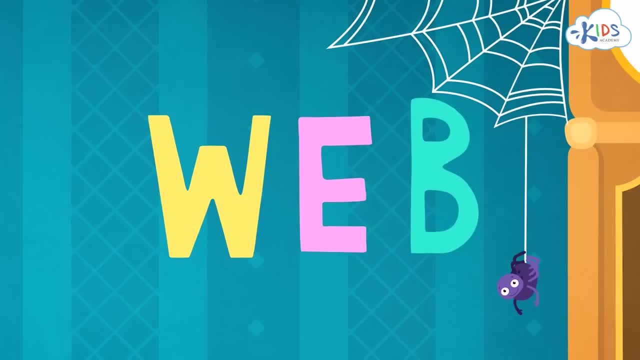 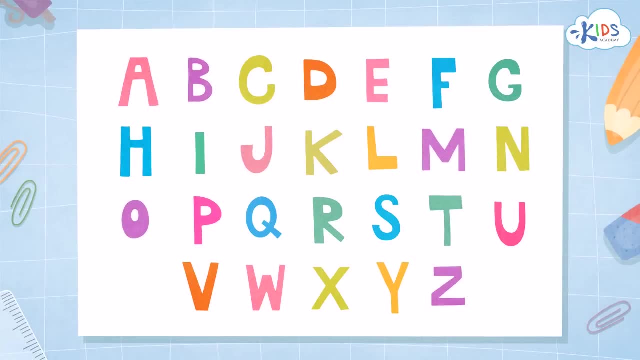 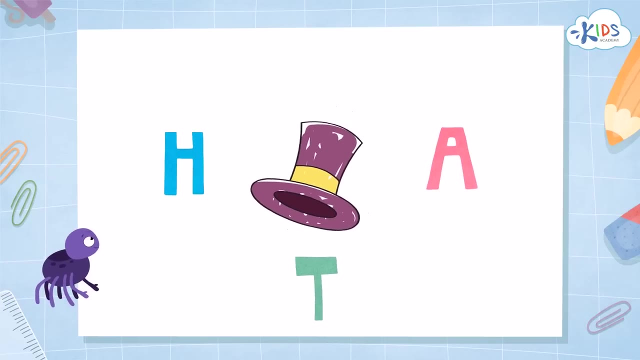 we have our word w- e- b- web. Let's practice putting letters in order to make a word together: H, T, A. These letters are in the word hat, but they are all out of order. Let's see if we can figure out the. 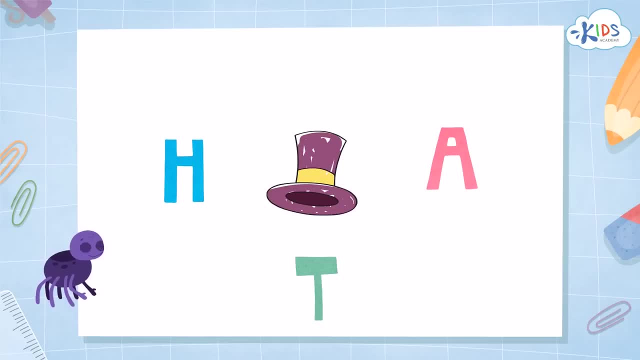 letters to make the word hat. The letter H makes the H sound. The letter T makes the ppbe sound. The letter U sounds like h t e s. The letter T makes the r " t sound. The letter A makes the a sound. The word hat starts with the h sound. It is the. 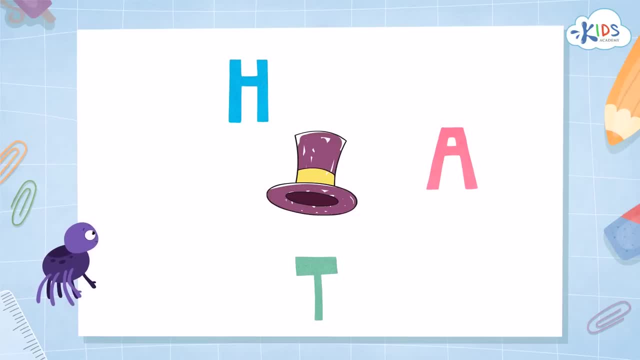 letter H. The word hat has the a sound in the middle. That sound is the letter A. The word hat ends with the t sound, The letter T Hat. Now you can practice putting letters in order to make words on your own. Bye. 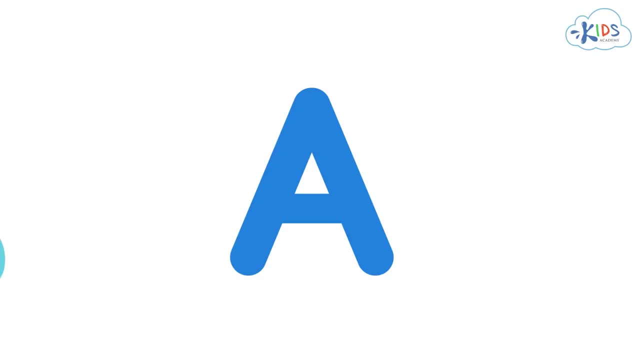 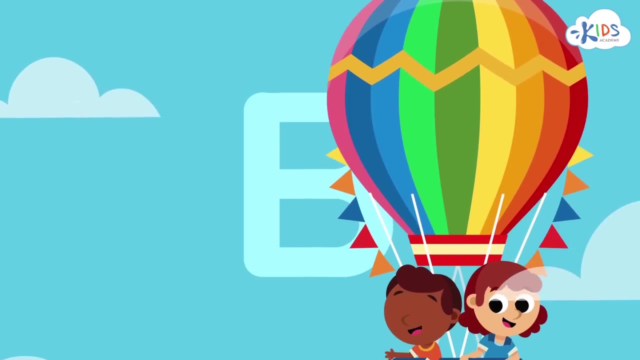 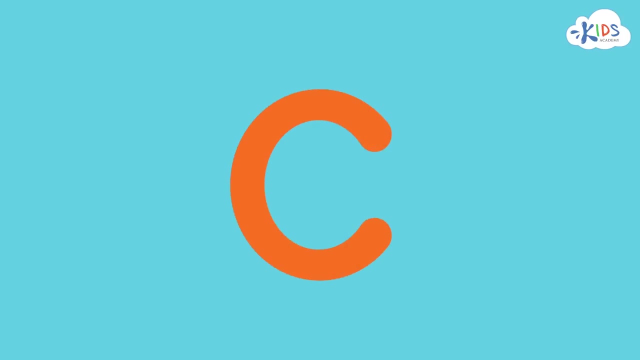 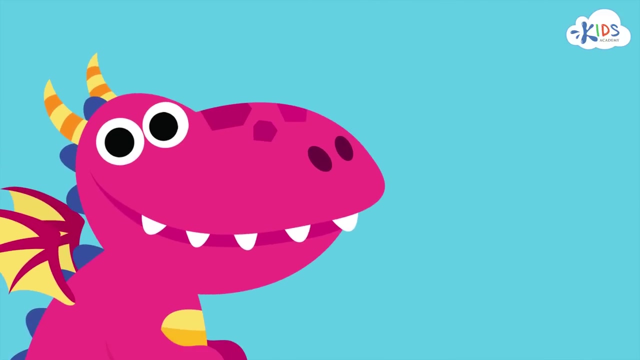 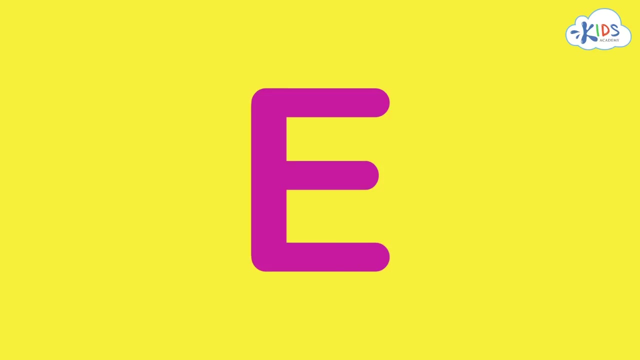 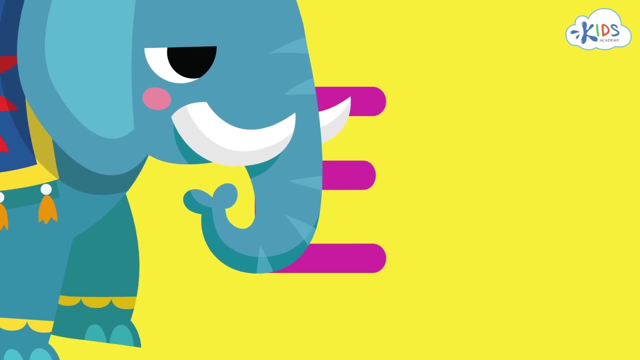 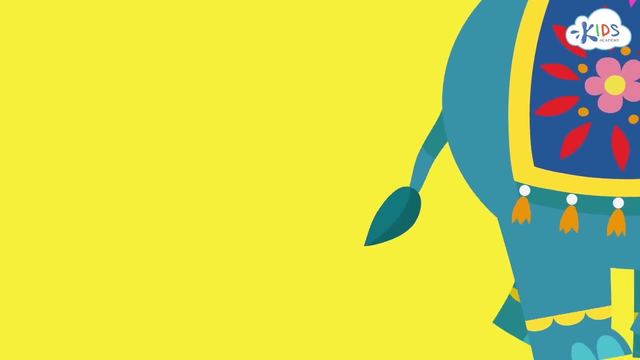 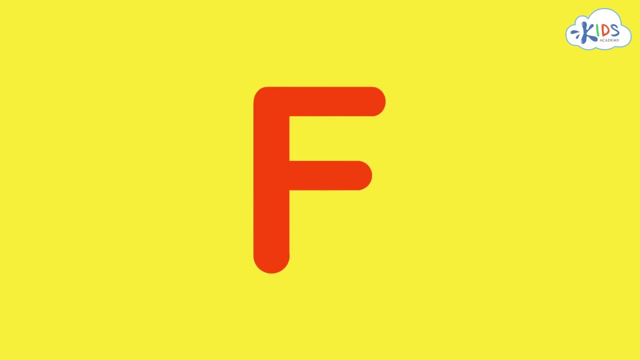 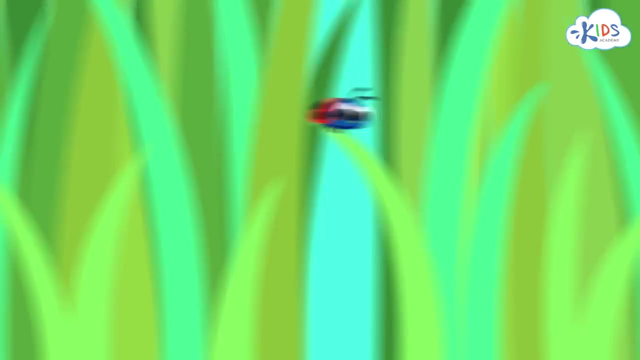 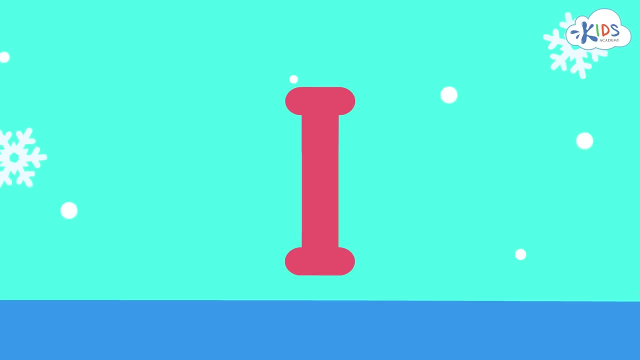 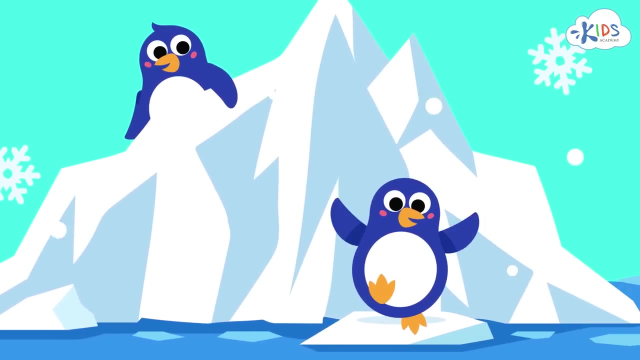 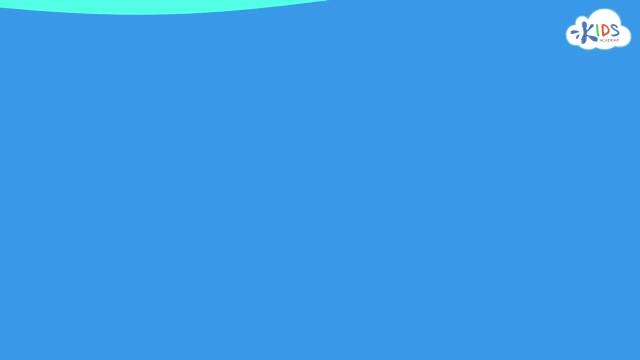 Upper case A. Upper case B. uppercase C. uppercase D. uppercase E. uppercase G. uppercase D. uppercase F. uppercase F. uppercase G. uppercase G. uppercase G. Uppercase H. Uppercase I. Uppercase J. Uppercase K. Uppercase L. 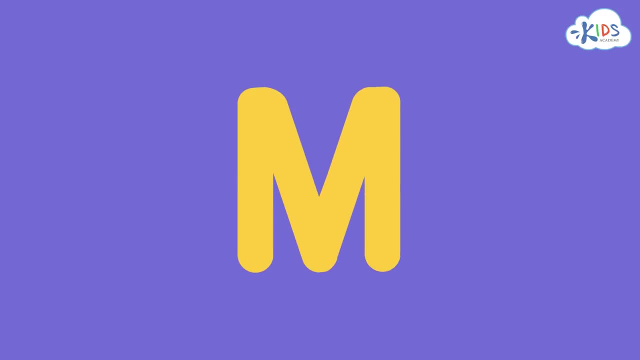 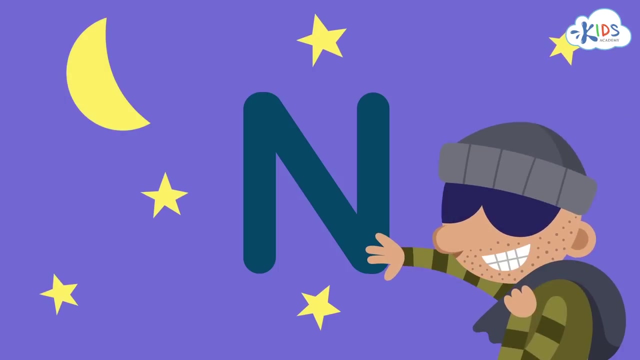 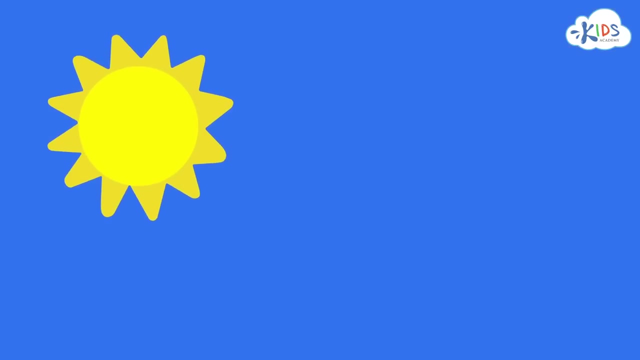 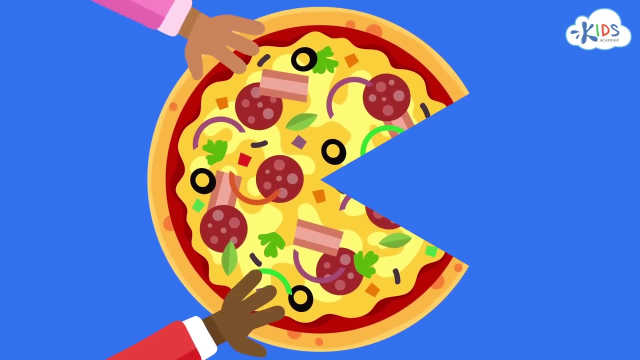 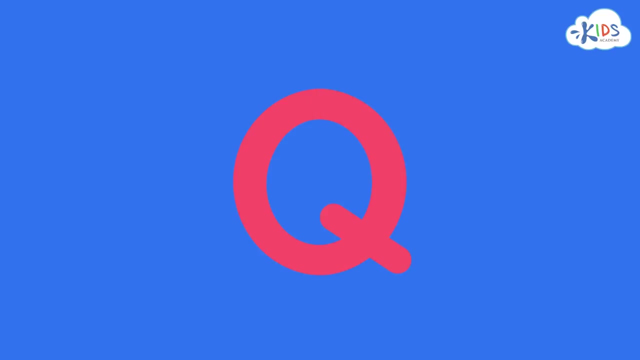 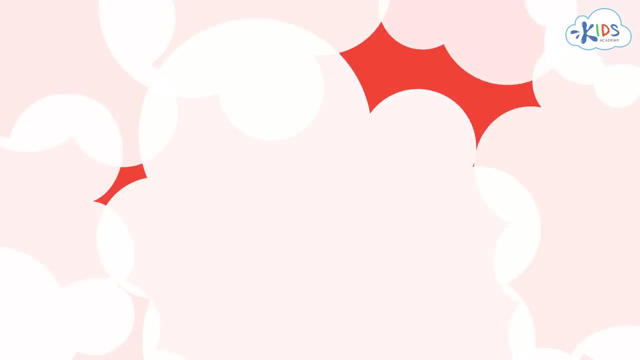 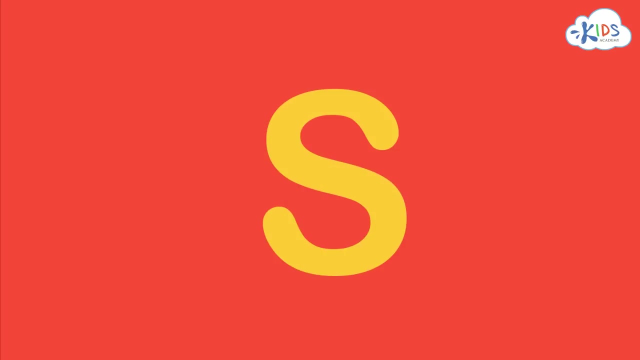 Uppercase M. Uppercase N. Uppercase O. Uppercase P. Uppercase Q. Uppercase R. Uppercase S. Uppercase T. Uppercase U. 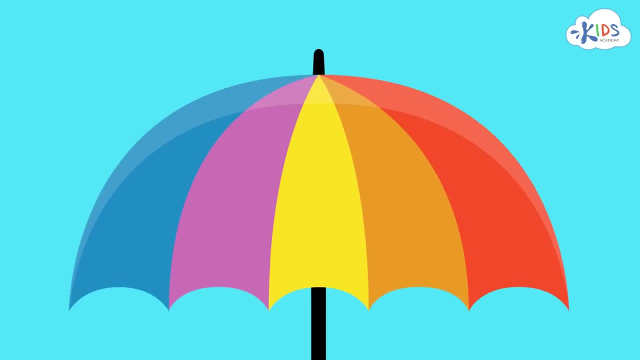 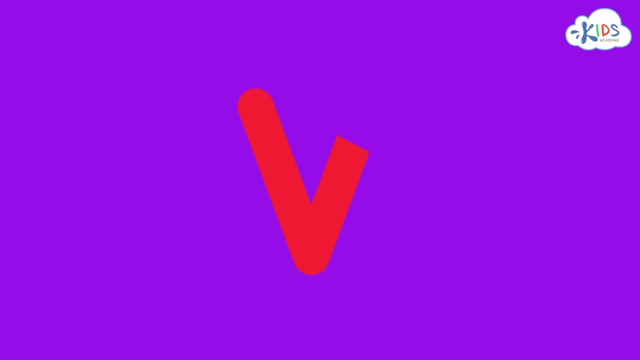 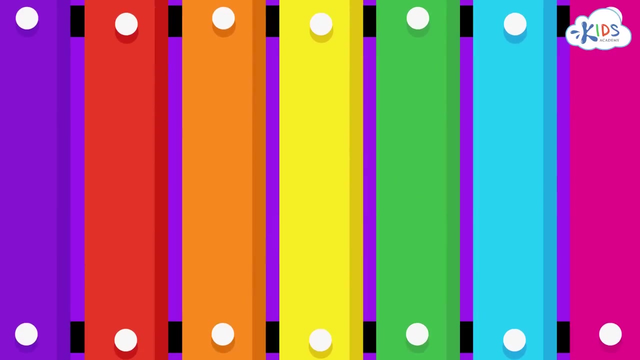 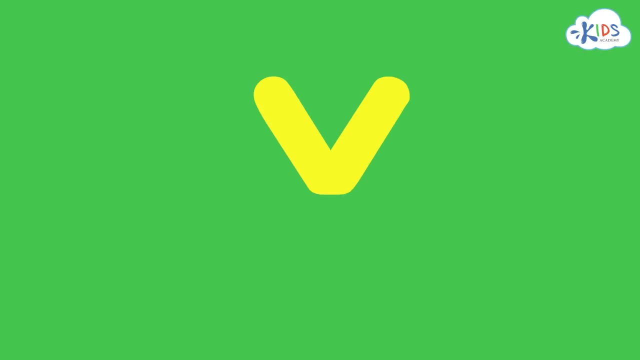 Uppercase V. Uppercase V. Uppercase W. Uppercase X. Uppercase Z. Uppercase Y. Uppercase Y. Uppercase Y. Uppercase Z. 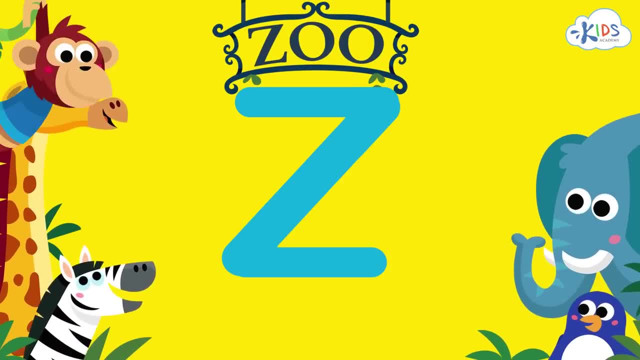 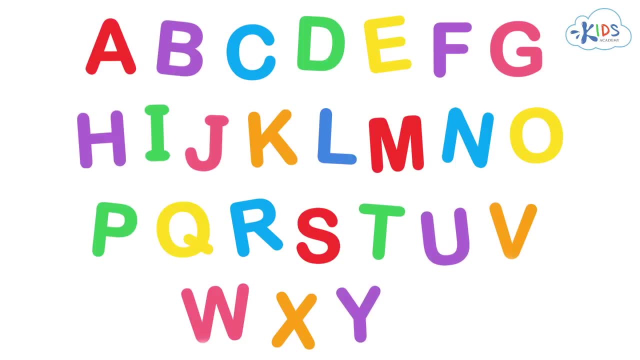 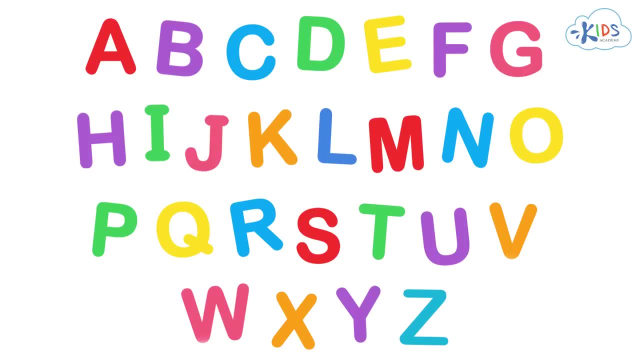 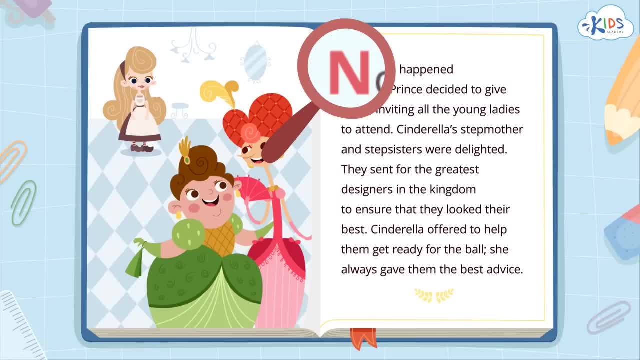 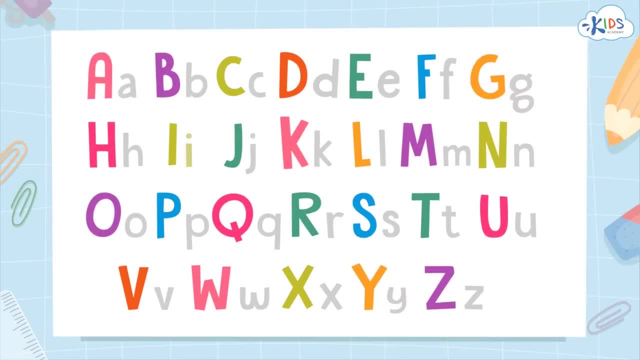 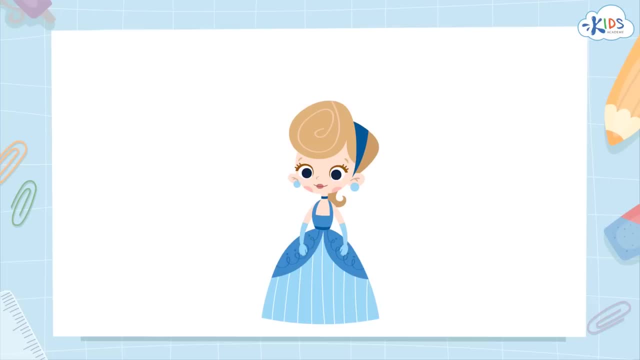 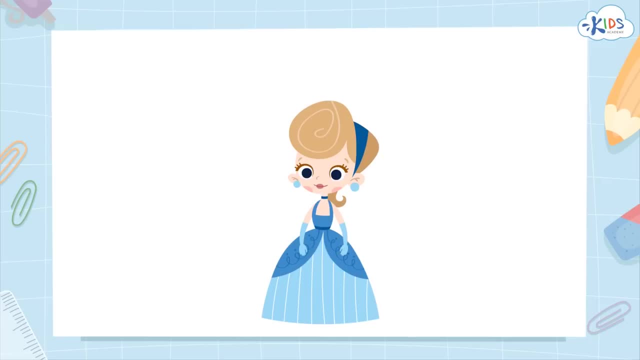 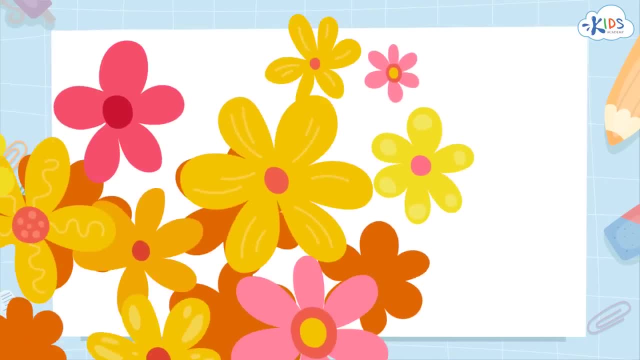 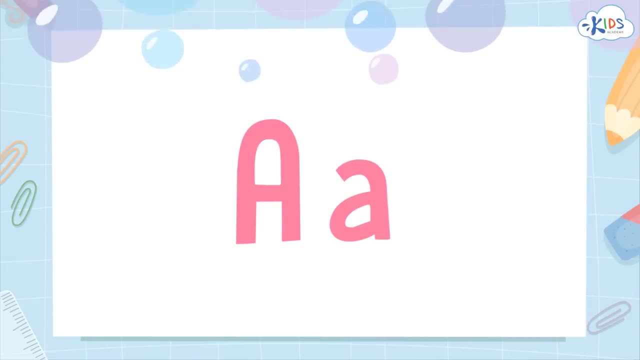 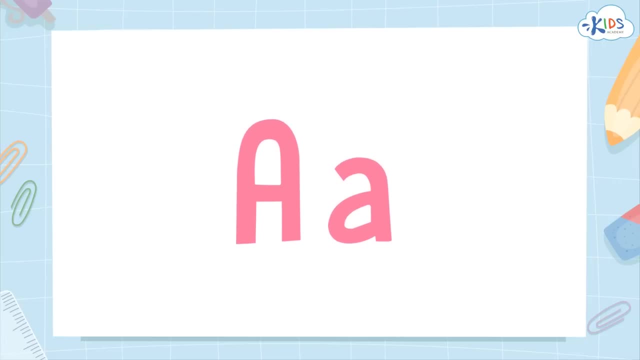 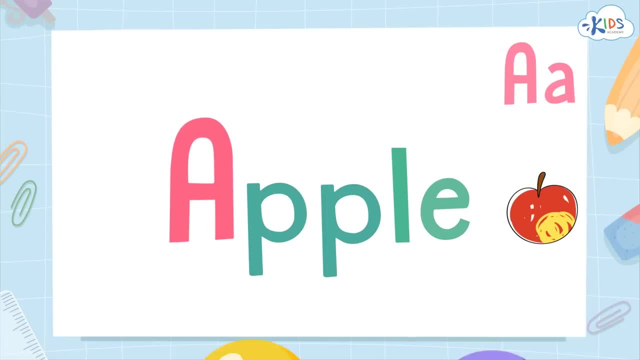 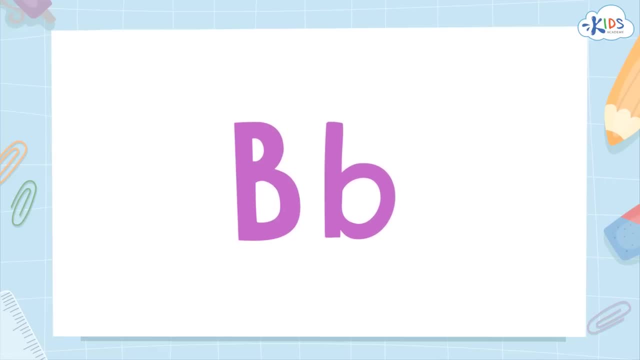 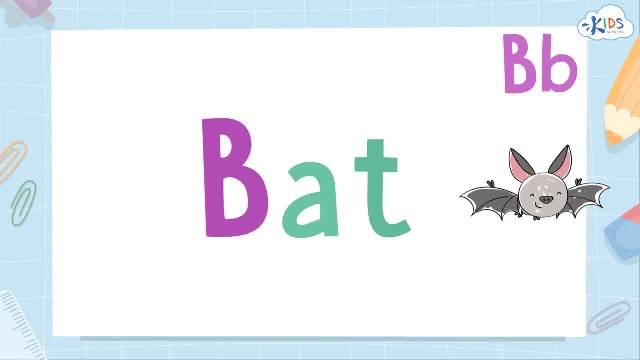 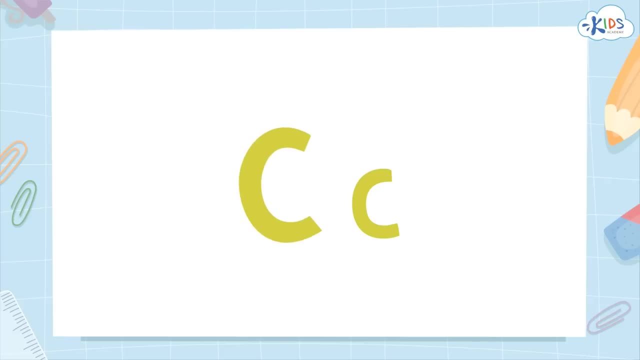 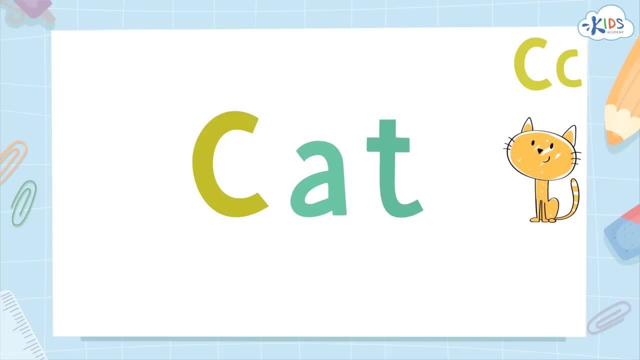 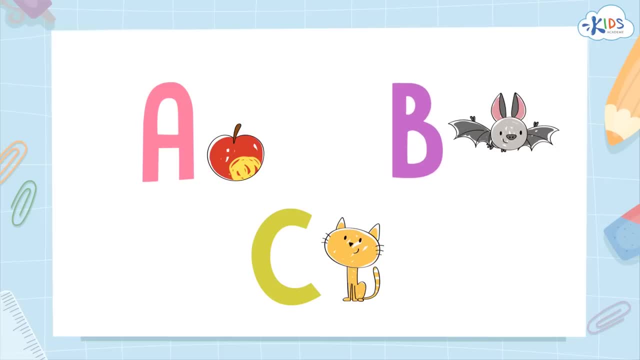 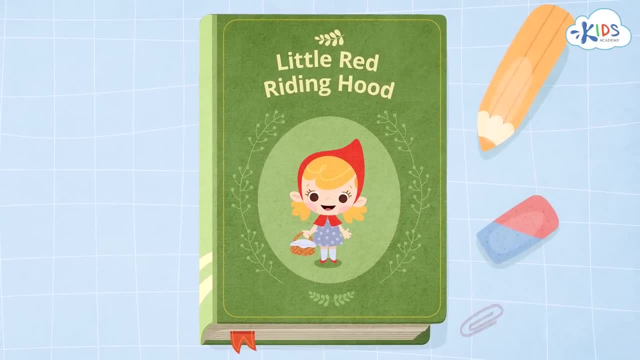 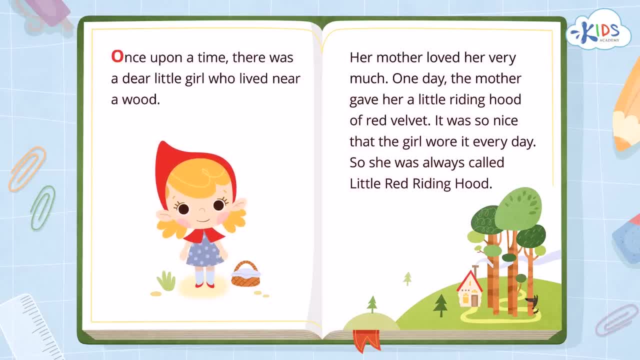 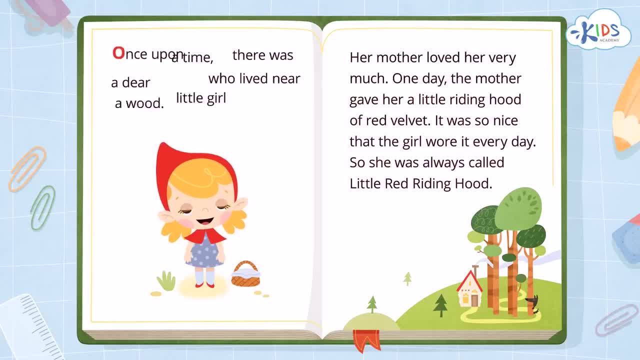 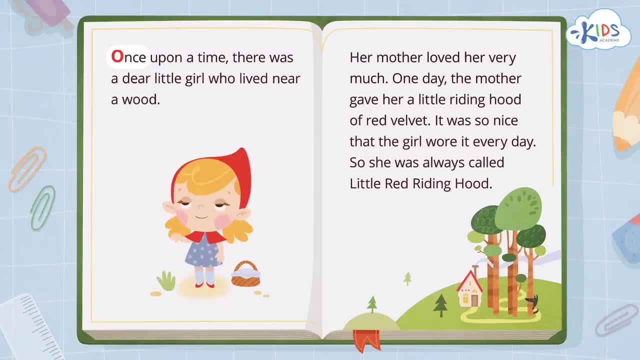 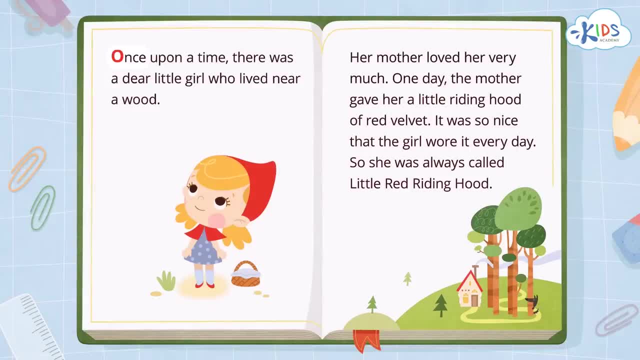 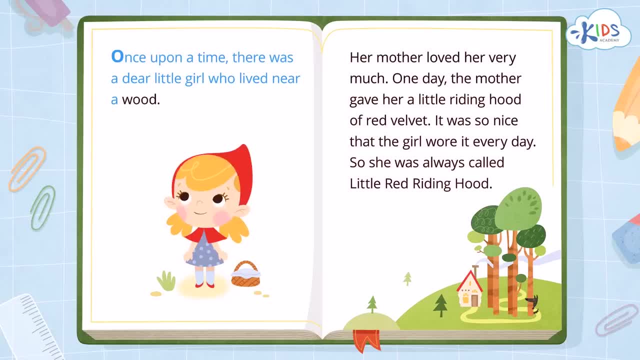 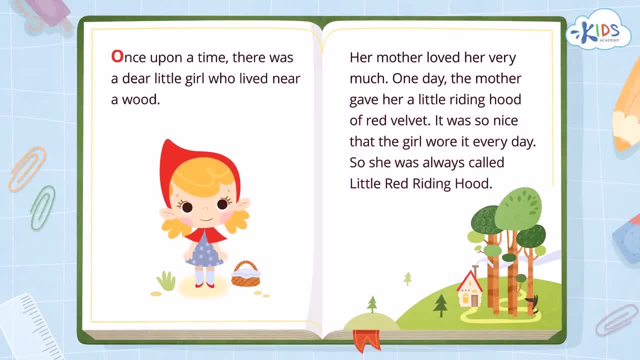 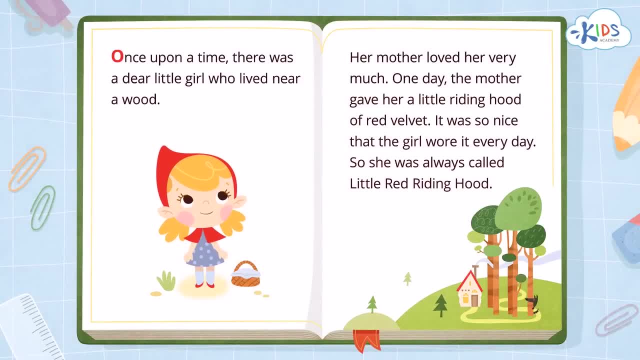